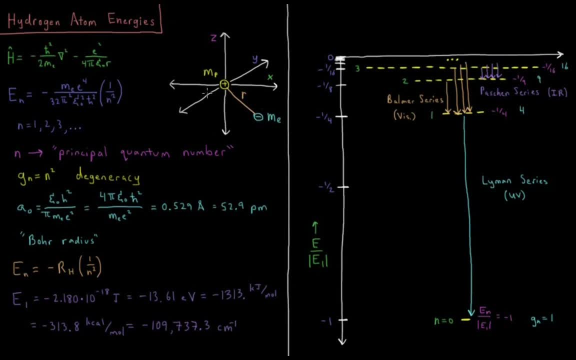 away from the proton. The electron is free to go anywhere in three-dimensional space, in x, y and z, but for reasons of convenience and because of how our potential energy function works, we have preferred to write our wave functions in terms of spherical polar coordinates, r, theta and 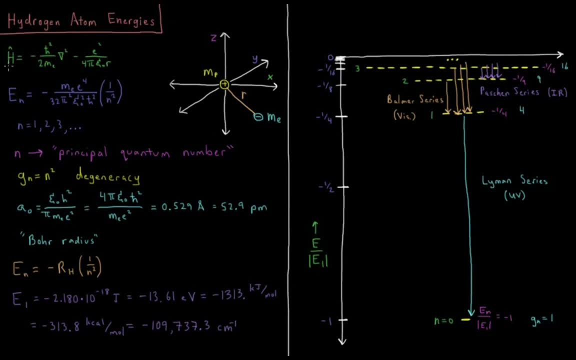 phi. So our Hamiltonian from the previous video is equal to minus h bar squared over two times mass of the electron times del squared, the Laplacian operator, minus e squared over four pi. epsilon naught r, the Coulomb potential Energy this electron feels due to the presence of the proton. We are using the mass of the electron. 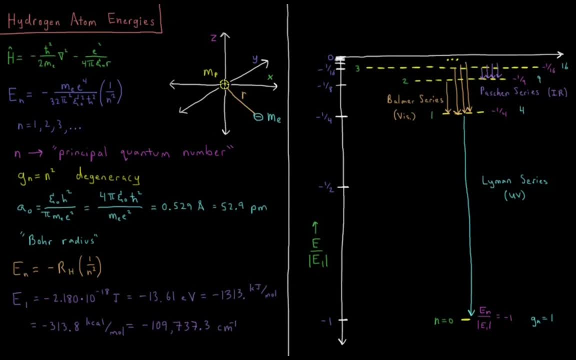 here instead of the reduced mass of the system, because we're assuming that this proton is just fixed at the origin and that the proton doesn't move. So what are the energy levels of this system here? So they depend on a quantum number, which we're going to call n, as we so often have for 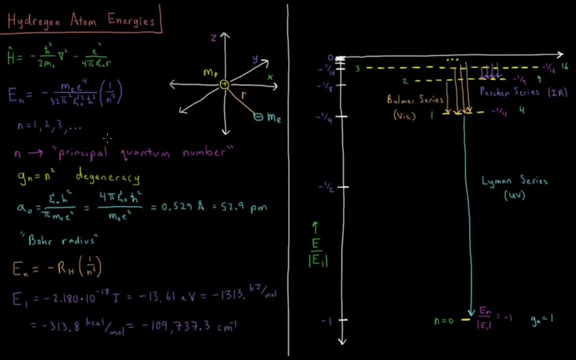 our model systems. n starts at one and it goes up to infinity and it is an integer. It's also referred to as the principal quantum number of the hydrogen atom. So the energies equal negative mass of the electron times magnitude of the charge of the electron to. 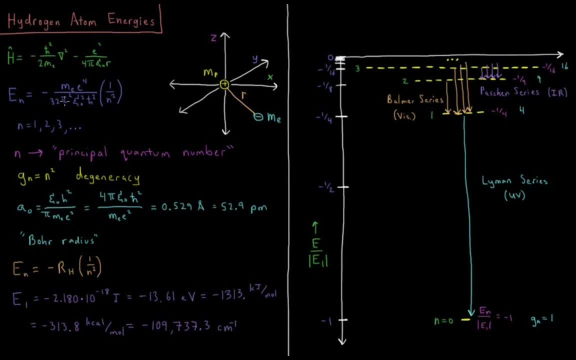 the fourth divided by 32, pi squared, epsilon naught squared. permittivity of free space squared, h. bar squared. Planck's constant over 2, Pa quantity squared times 1 over n squared. So those are our energy levels. We can see those over here. 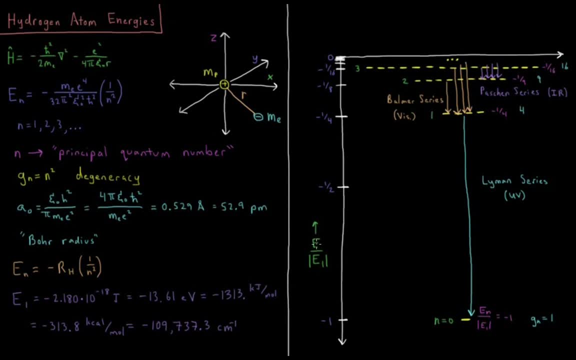 So the lowest energy state. if we use units of E over E sub 1, that's going to be at minus 1 there. Then our energy depends on 1 over N squared from there. So E2 is going to be 1 fourth times E1.. 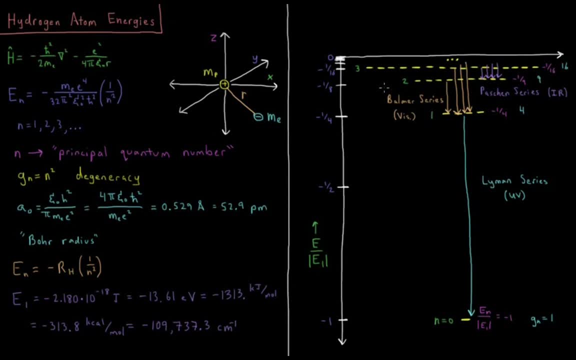 E3 is going to be 1 ninth times, that E4 is going to be 1 sixteenth. I have these quantum numbers mislabeled, so I'm going to fix that right now, Much better. So 1 ninth for N equals 3 relative to the original N equals 1 level. 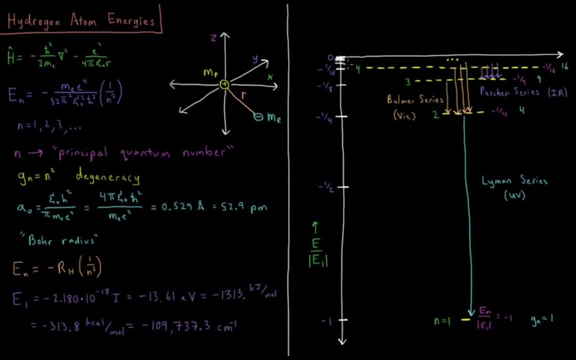 and 1. sixteenth of that, approaching all the way up to the zero in energy. We also have degeneracy in this system. The degeneracy of a given energy level of this principal quantum number is equal to N squared. So for N equals 1, we have 1 energy level. 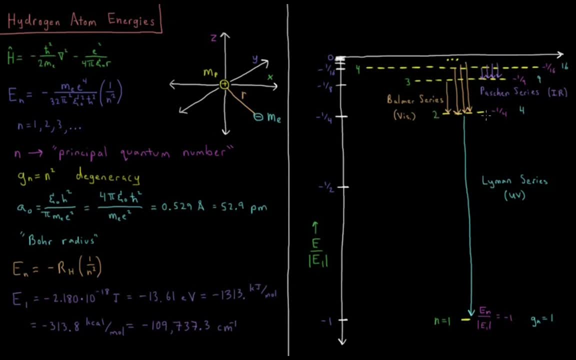 For N equals 2, we have 2 squared or 4 states. N equals 3, we have 9 states, N equals 4, we have 16 states, And after that it becomes very difficult for me to draw, so I stopped. 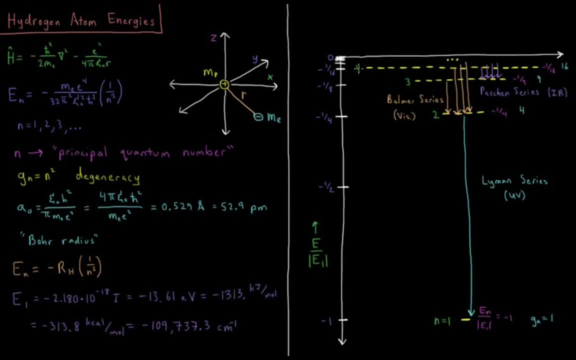 So you can use your imagination for states beyond N. equals 4 for that N squared level of degeneracy. Alright, so we have. Let's remind ourselves of the quantities. Let's see the Bohr radius here, So that equals epsilon naught Planck's constant squared over pi times mass of the electron, times magnitude of charge of the electron squared. 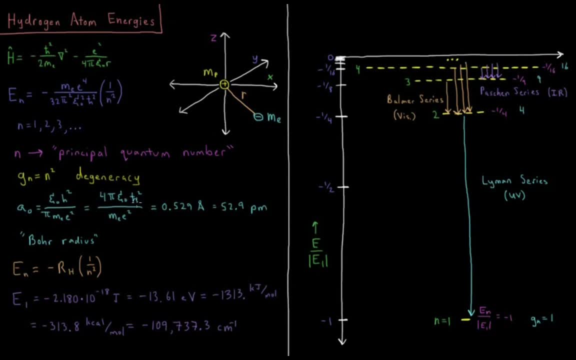 So that's equal to 4 pi. epsilon naught h-bar squared over m-e. e-squared was also equal to 0.529 angstroms, or 52.9 picometers, 1 angstrom being 10 to the minus 10th meters. 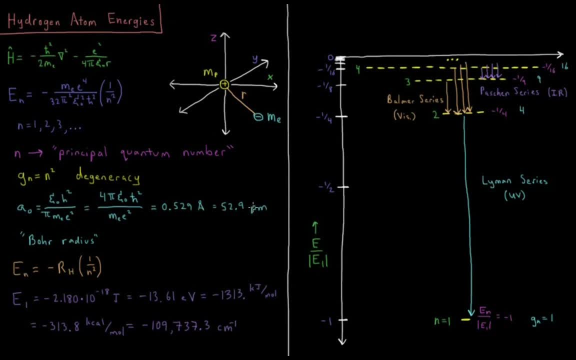 1 picometer being 10 to the minus 12 meters, 1 trillionth of a meter. Not sure why I put that there, but okay, that's fine. The energy is also equal to the negative value of the Rydberg constant times 1 over N squared. 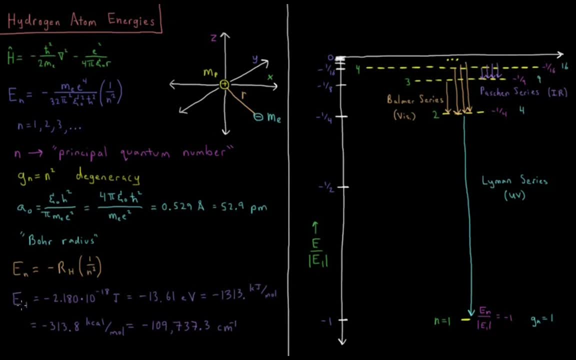